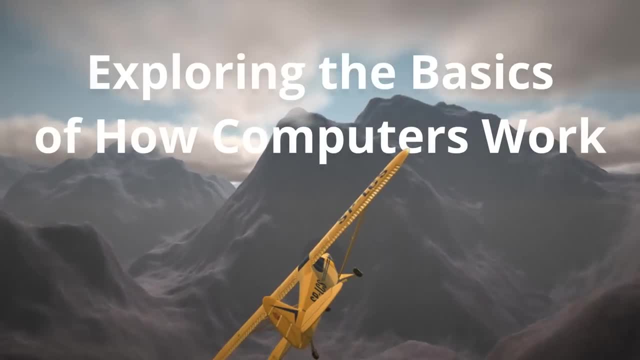 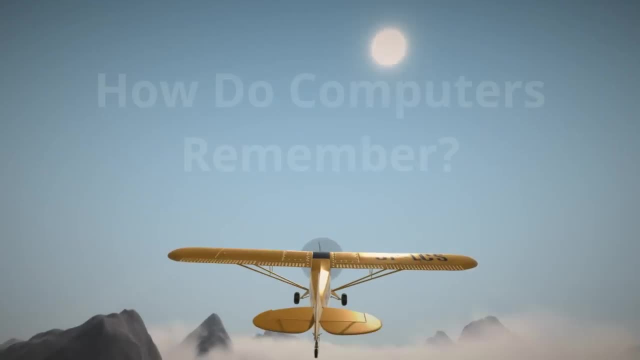 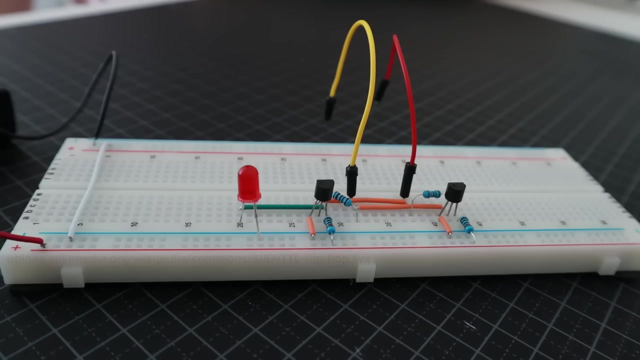 that it's working with, So I've begun by creating this simple circuit following a little diagram I found online. If I take this red wire and connect it up here, the light turns on. What's interesting, though, is if I then take the wire back out, the light remains on. 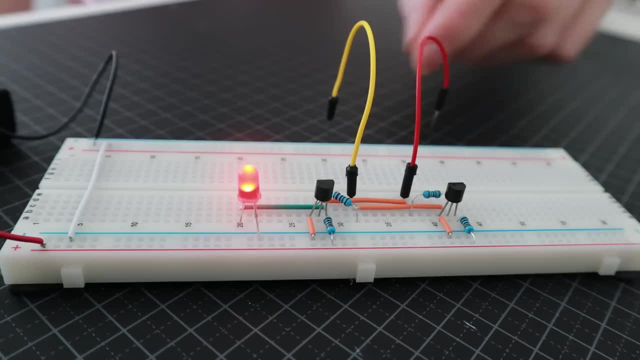 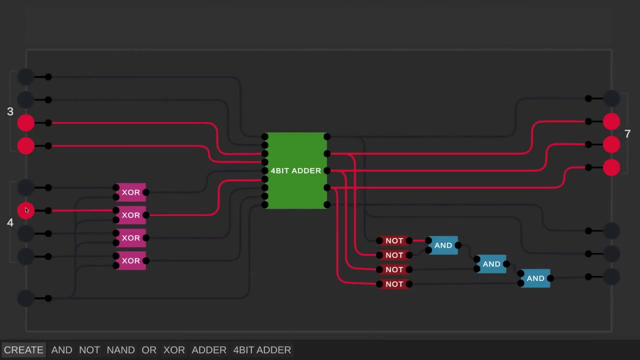 So somehow the state has been remembered. The other wire, by the way, can be used to turn the light back off, and so we can think of these two wires as being the set and reset inputs to our circuit. Let's switch over to the little simulation program, where we managed to get addition and 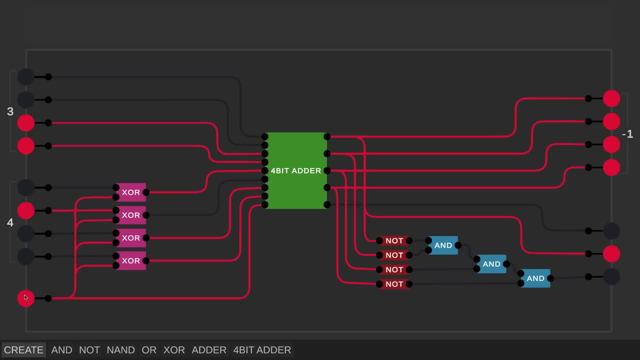 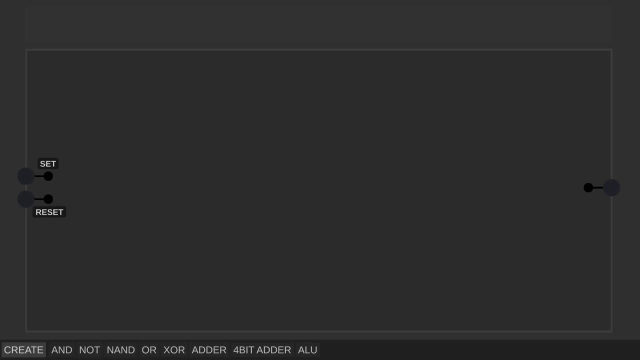 subtraction working last episode and try create some of this mysterious memory. So I have our two input signals here, set and reset, and together these should control the state of the circuit. One way we can achieve the behaviour we saw is using an AND gate, an OR gate and a NOT. 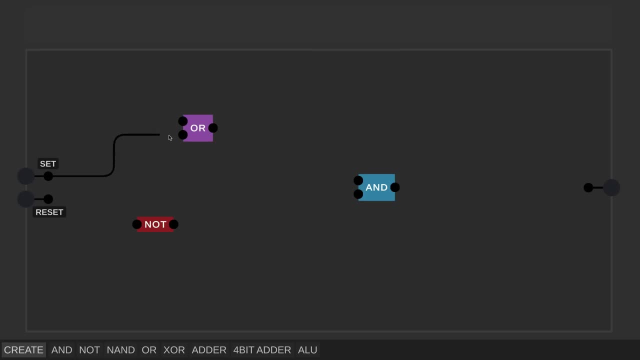 gate, The set input goes into the OR gate and the reset input gets inverted and then goes into the AND gate and you can see the signal travelling along there. Now the output of the OR gate goes into the AND gate as well, and the result of that is: 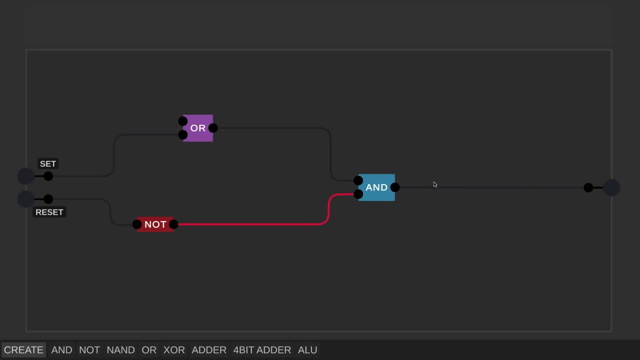 our final output signal. But now for the fancy part. this output signal gets fed back to the OR gate. Let's see how this behaves. So I'll turn on the set input which makes the OR gate turn on, which makes the AND gate turn on, and so now our output is on. 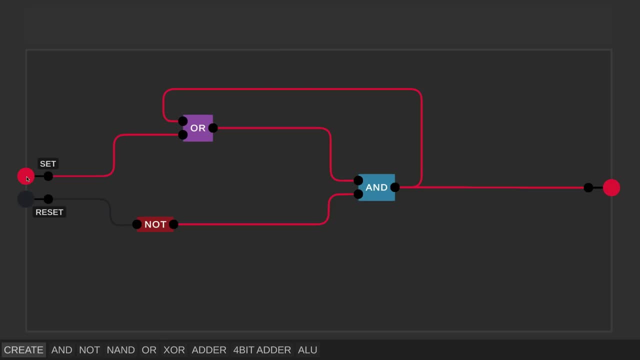 Of course this has also turned on the other input to the OR gate. so even if I now turn the set signal off, the output remains on. The only way to change the output now is using the reset signal, so let me try turning that. 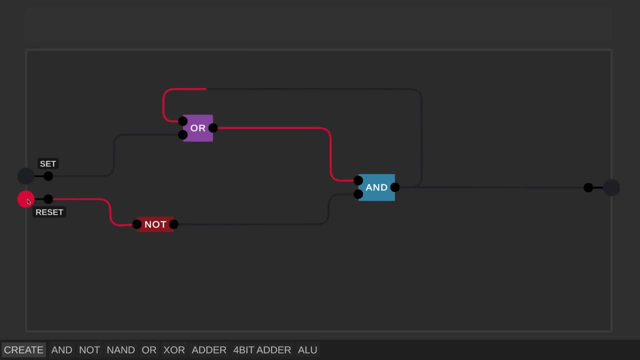 on. This signal is inverted, so it turns off the input to the AND gate. Now let's look at the output, So we can see that the set signal has turned off and the to the AND gate, and so the output switches off as well. I can now turn the reset input off. 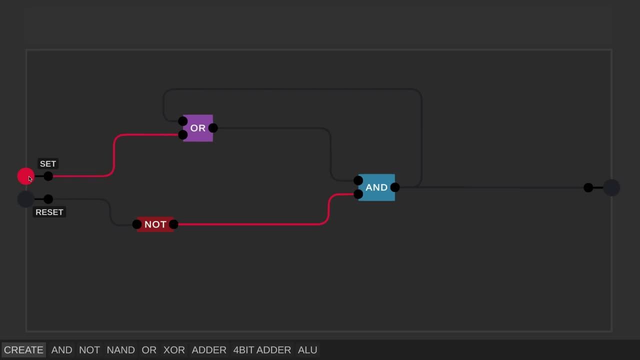 and the output will stay off. This little setup is known as a set reset latch- SR latch for short. I'd like to look at a different way of constructing this latch, which I think is really interesting. but first I'll need a new building block, which is an OR gate, followed by a NOT gate. 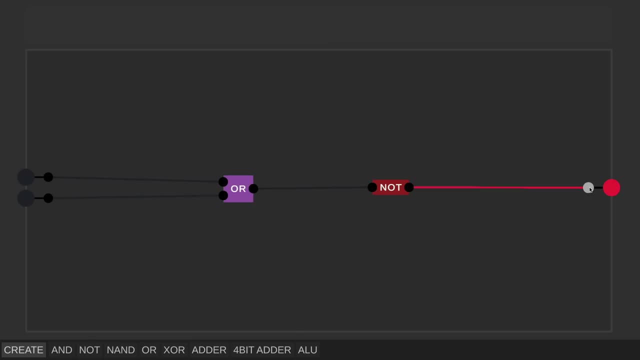 making what's called a NOR gate. Here the output is only on when both inputs are off. so if I turn either of these inputs on, the output will switch off. I'll write its name up here and then make it into its own little chip. 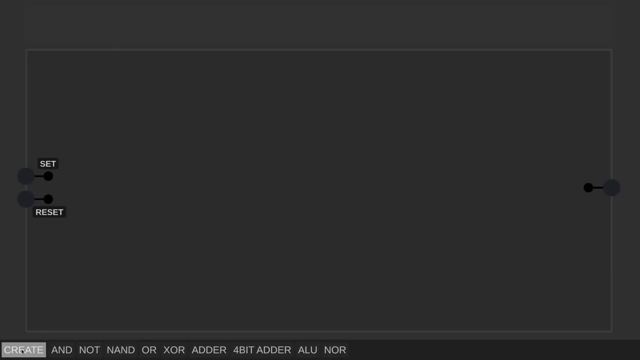 Okay, so here we have our set and reset inputs once again, and what I'll do this time is take two of the NOR gates and feed the output of the first one into the input of the second. Both inputs of that first NOR gate are unconnected, which the simulation just treats as off. 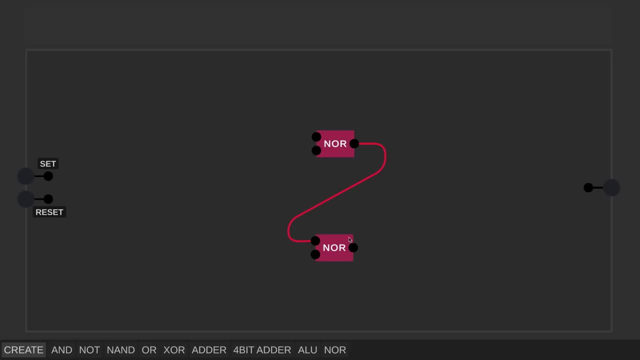 and so its output signal is currently on. This will cause the output of the second NOR gate to be off, and I'll wire that up to the input of the first one. I'll also connect it to the output signal over here and finally, I'll hook up the set and reset inputs like this: 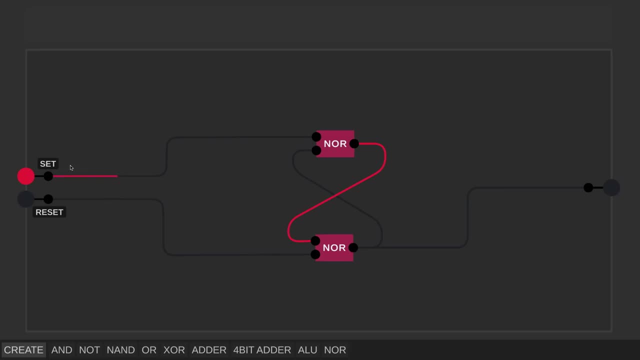 So let's try turning on the set input, which will make the output of this NOR gate turn off, which then makes the other NOR gate's output turn on, and so our output signal here goes on. We also have this signal travelling along here. 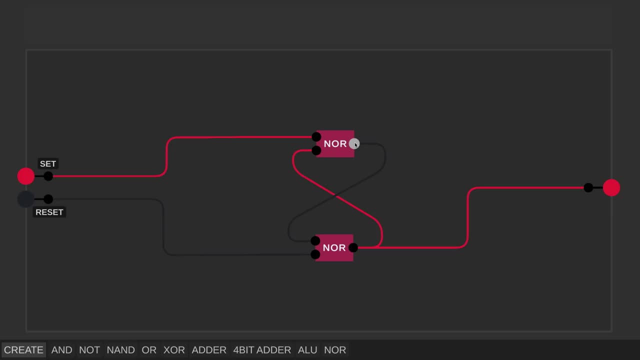 which we can think of as essentially locking this output into an off state so that it remains off even if we now turn the set signal off. And so, as you can see, the output here has remained on. Let's try turning on the reset signal now, so this will switch off the output of this NOR gate. 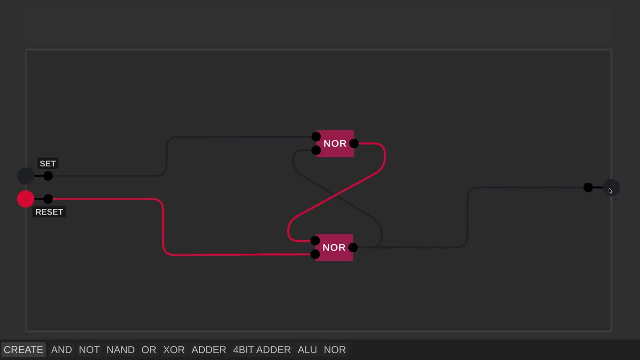 and, as a result, the output signal here will go off. That also means that this signal along here is now off, allowing this output to come back on, which again locks the output of this NOR gate into an off state, so that even if we turn the reset. 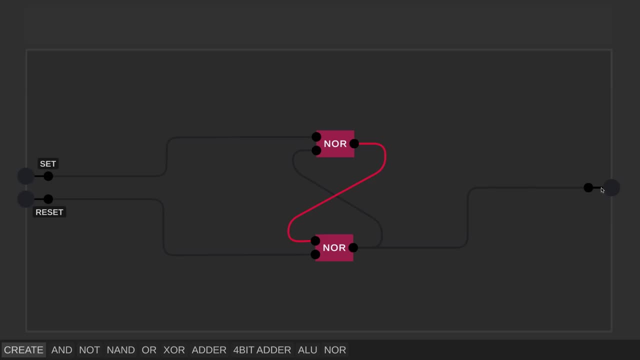 signal off. the output remains off. This setup looks really simple, but it can definitely take a little while to wrap your head around what's going on here. Anyway, what I'd like to do next is modify this slightly so that, instead of having a set and 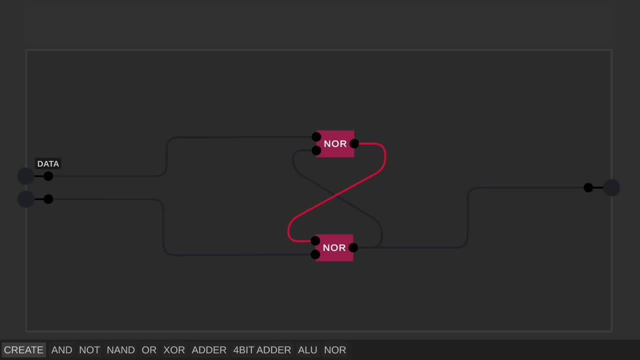 reset input. we have an input for data and a store signal which indicates whether we want to save that bit of data or just ignore it. To make this work, I'll need to remove these two wires and add in two AND gates. 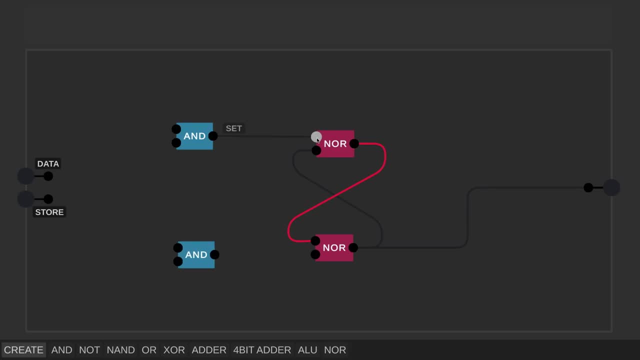 The output of the first gate will play the role of set and the output of the second gate will play the role of reset. So we want this set signal to turn on if we're sending a 1 on the data signal and the store signal is on. 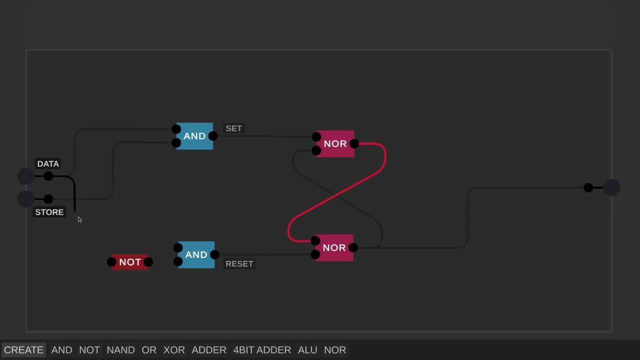 And we want reset to go on. if we're sending a 0 on the data signal, so I'll need to invert it to test for that and once again the store signal is on. So if I now put a 1 on the data input, nothing really happens until I enable the store signal. 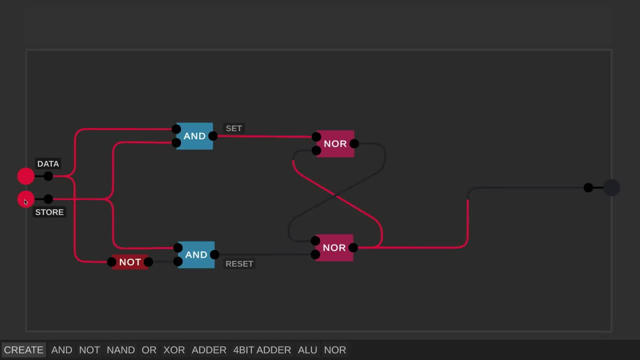 and now we should see the output change to a 1.. If I then turn the store signal off, I can again change the data to my heart's content without it having an effect on the output. As a final test- with the data now set to 0, I'll enable the store signal again. 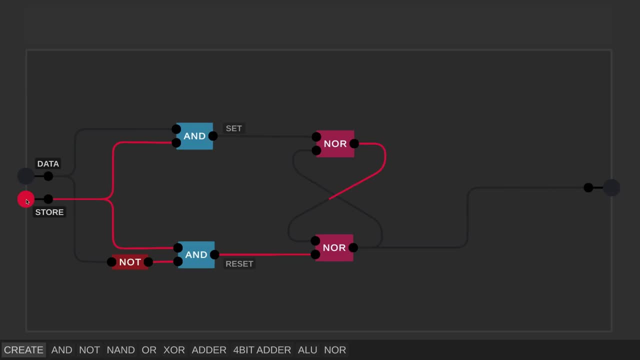 and we should see the output now change to 0.. So this started out as a simple test, but now we can see that it's working. started out as a set reset latch, but after a little modification I'll call it a data. 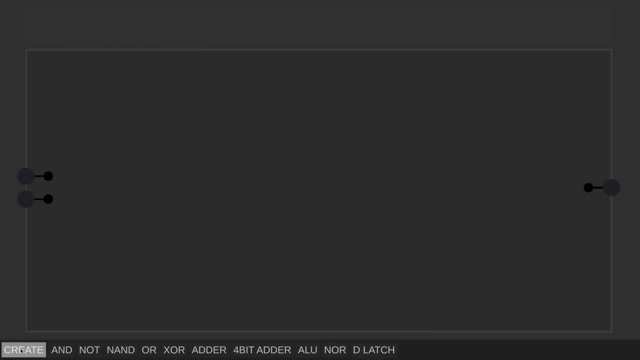 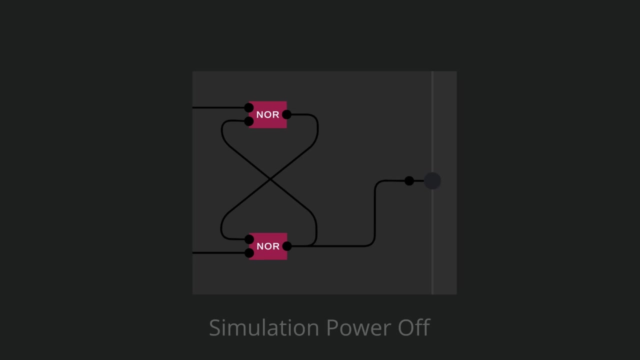 latch. instead, Let's take a moment to consider this core part of the latch in particular: what happens when the power is off? so the simulation is unplugged, so to speak, and we then turn the power on. It's interesting because the inputs to both NOR gates will initially be off, so both of 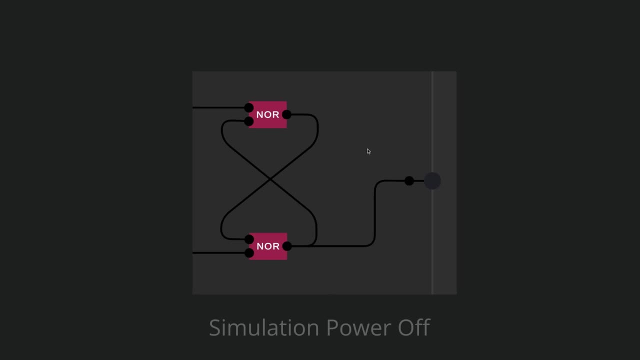 their outputs will be on. As you can see, I get this weird oscillating effect in my simulation, where the output endlessly toggles on and off. I was confused at first about why this wouldn't happen in real life, but I think I roughly 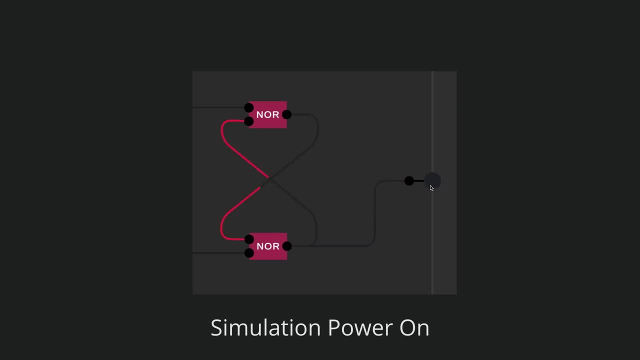 understand it now. The signals in the wires are travelling really fast, somewhere in the vicinity of half the speed of light. What's much slower- although we're still talking nanoseconds- in reality is something called the gate-displacement. This is how long it takes for the output of a gate to fully react to a change to its inputs. 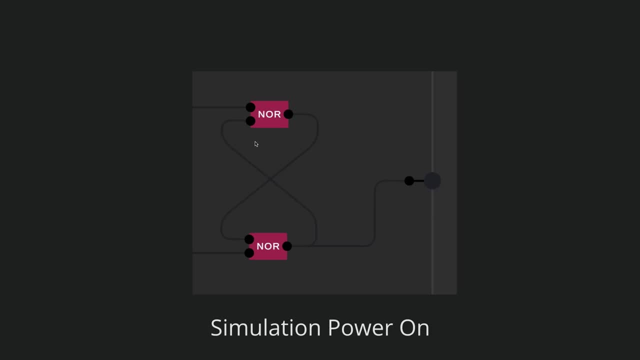 So I guess that it looks something like this. But now small variations in the gate delay will result in one of the signals getting to the other gate first, preventing it from outputting anything like. so I'll restart this and we can see it settled into an on state. I'll restart again, and this time it happened to settle into an off state. I was curious to try this out with that little srlatch I built earlier and, sure enough, sometimes the light was on initially and sometimes it was off. 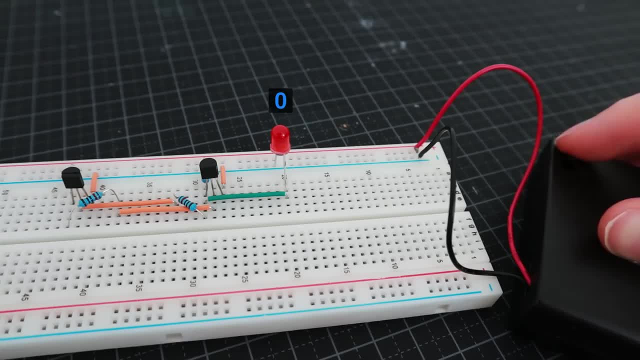 So the start state is essentially random, although it might heavily favour one state over the other, I guess, because one of the gate delays could just naturally be a little slower than the other. Anyway, I thought it'd be fun to try and replicate the exact setup we created in the simulation. 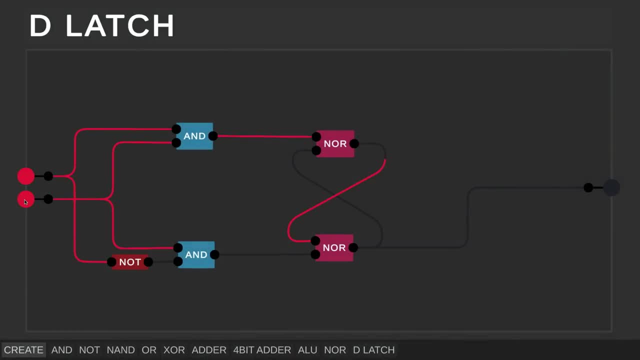 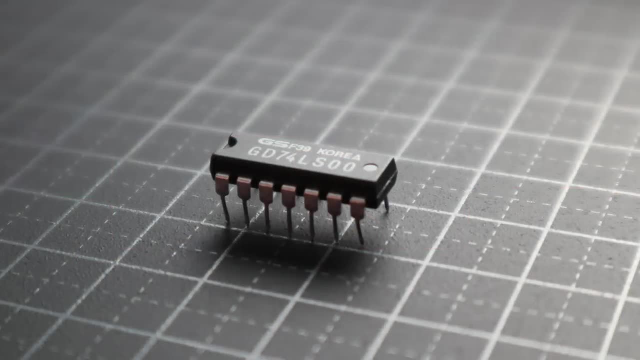 on the breadboard just to be completely convinced that it works in real life. Unfortunately, I don't have the time to do that. Unfortunately, I don't have any of these NOR gates AND gates or NOT gates. I do happen to own some NAND chips, however, and it just takes some small tweaks to get. 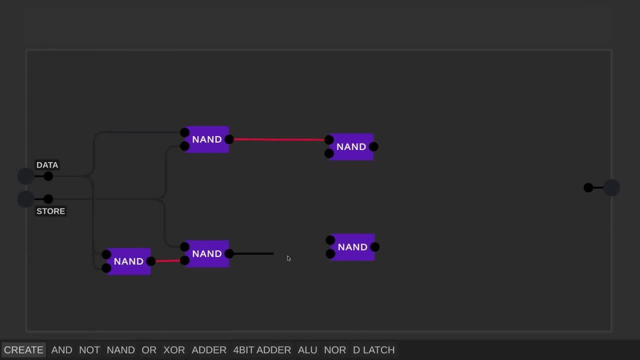 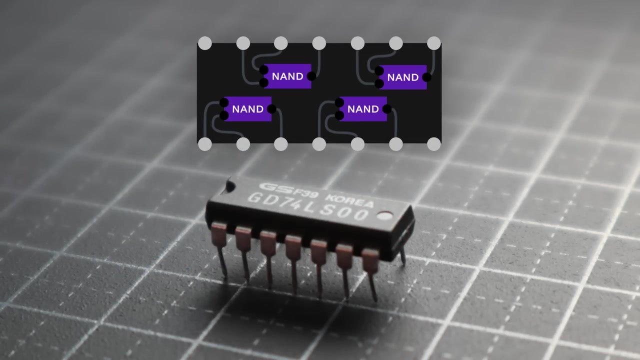 the same setup working in this simulation, made purely out of NAND gates like: so Okay, now each of these chips has actually got four NAND gates in total And, of course, unlike in my simplified simulation, real life requires everything to have a connection. 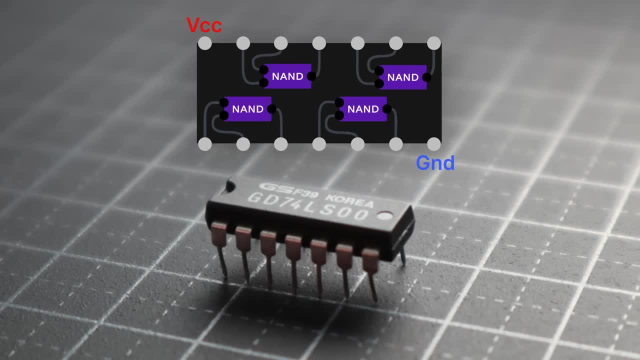 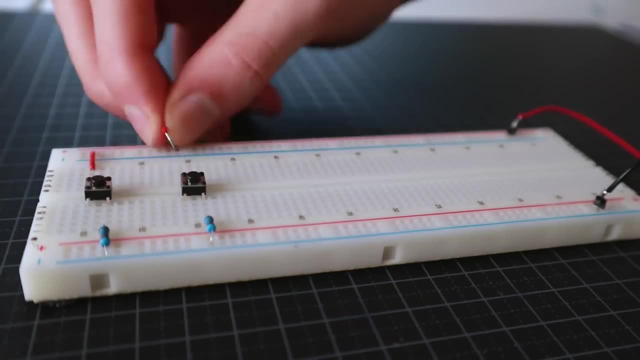 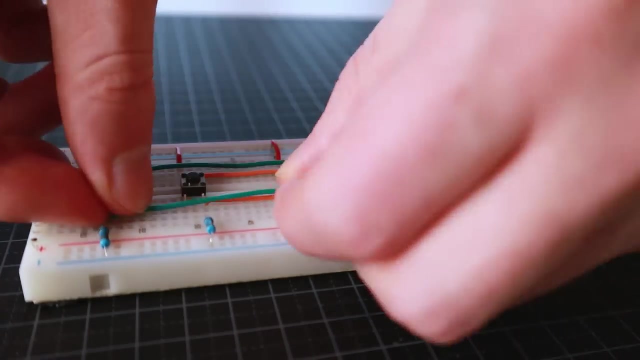 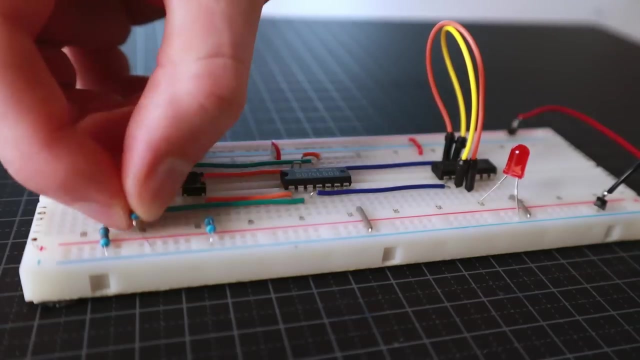 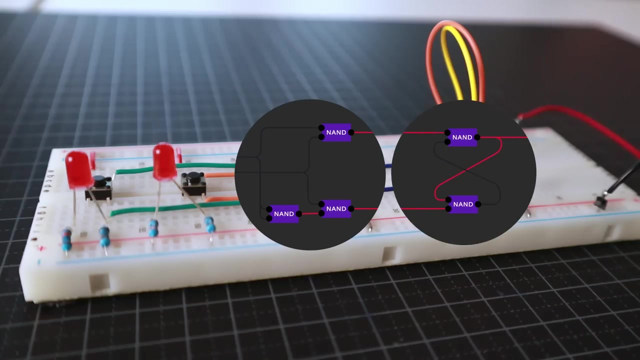 to power and ground in order to work. so that's what these other two pins are for. With that out of the way, let's start wiring this together. So I am using this first chip for these three NAND gates and the second one for these two. 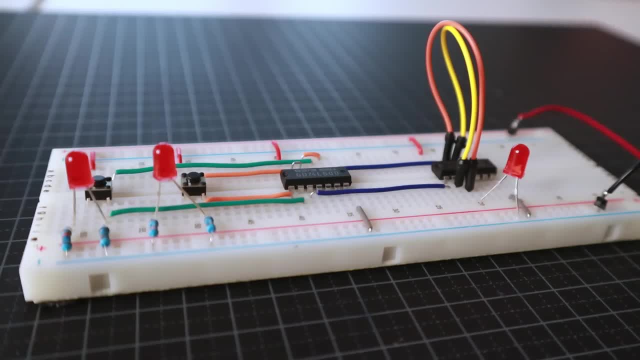 I probably could have set things up to use just one chip, but it seemed easier this way. Anyway, the little light on the left represents the store signal, then this is the data signal, and over on the other end is the output signal, and they're all currently zero. 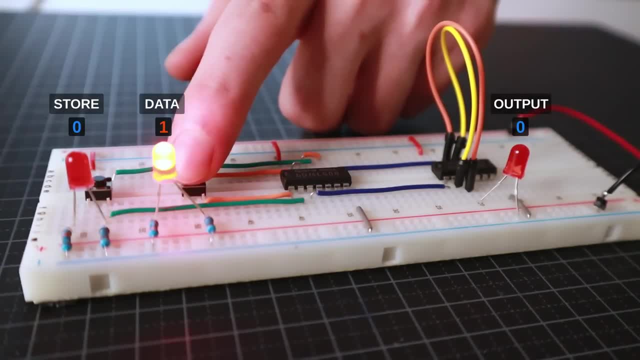 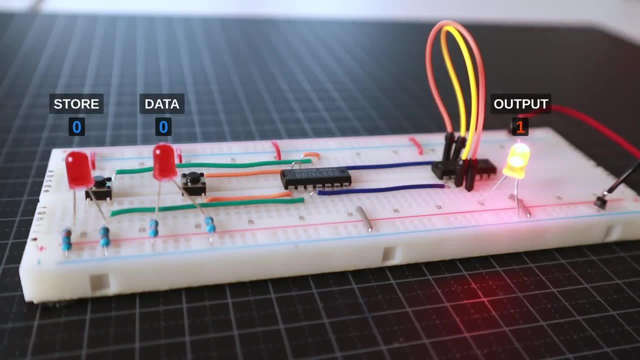 I can put a 1 on the data signal by pressing this button, But, as expected, the output doesn't change until I enable the store signal. so now the output is 1, and I can release the buttons and you can see it has remembered that. 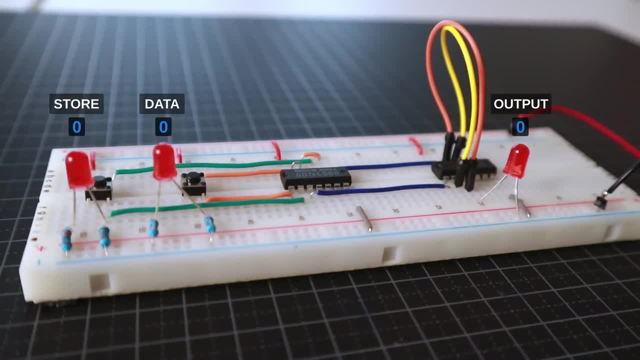 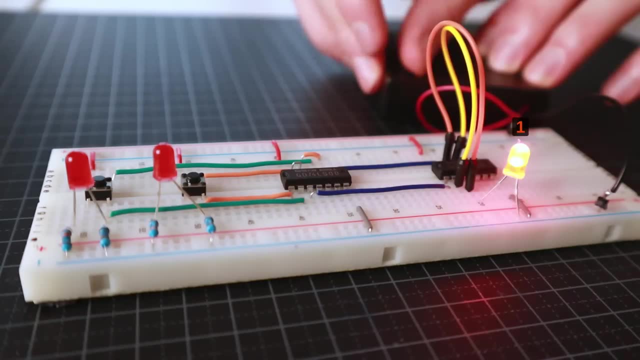 I'll then try storing a 0, and that seems to work as well. Last thing I'll do is just turn it on and off a few times to see what state it starts up in. I'm not sure why. I find this endlessly entertaining, but I do. 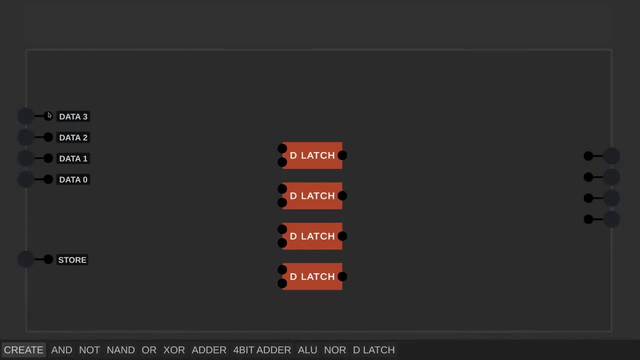 Okay, so with one latch we can store one bit of data, so of course we could just use four of them. if we wanted to store four bits of data, I'll quickly connect the store signal up to all of them and hook up the outputs as well. 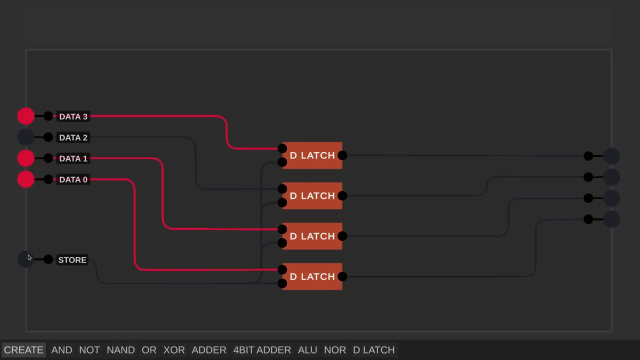 I can set some data but, as we're used to by now, the output doesn't change until the store signal is enabled. This is called a 4-bit register, but there are some potential problems with the current design and to understand them we need to think ahead to how these registers might be. 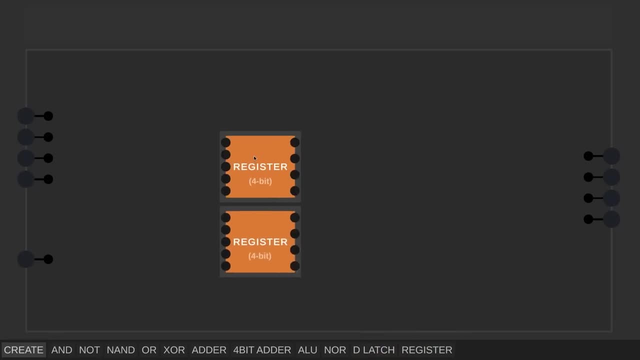 used. So, as an example, I'll take two registers. I'll creatively name A and B and I'll quickly connect these inputs up to A and store some initial value in there, say 3.. I'll then wire the inputs up to B instead and store maybe a 1 in there. 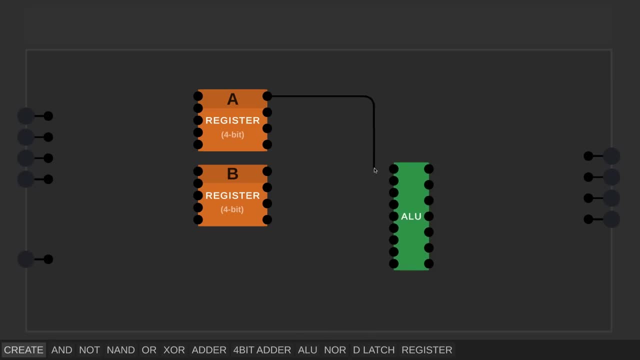 Okay, I'll now bring in the ALU we built last episode and connect the register outputs up to that. So at the moment the ALU should be adding the contents of the two registers together, since we don't have the subtract signal here enabled. 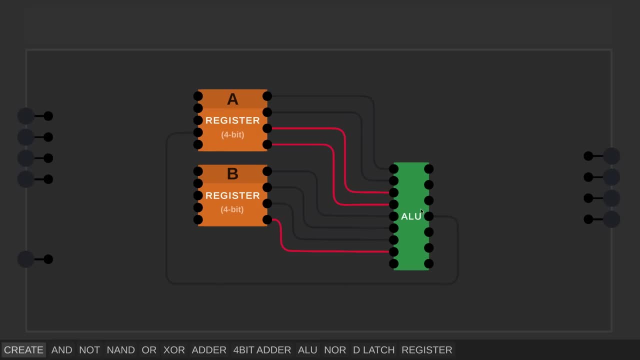 Now a pretty reasonable thing to want to do is take the result from the ALU and store it in the A register so we can use the result for whatever calculation we want to do next. By the way, we can see over here that the ALU is outputting 4,, like we'd hope. 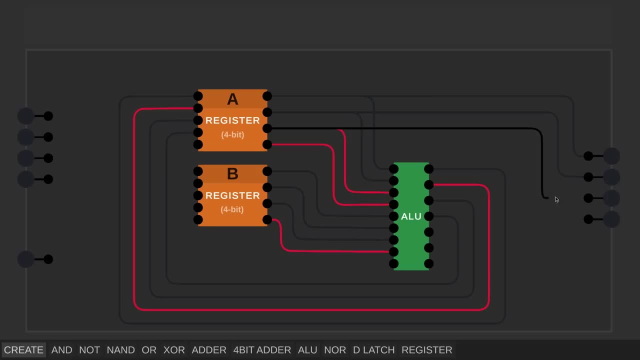 I'll quickly wire the A register up to the output signal so that we can see what value it contains. It's still 3, unsurprisingly so, to store the result from the ALU, we'll need to hook up the store signal over here. 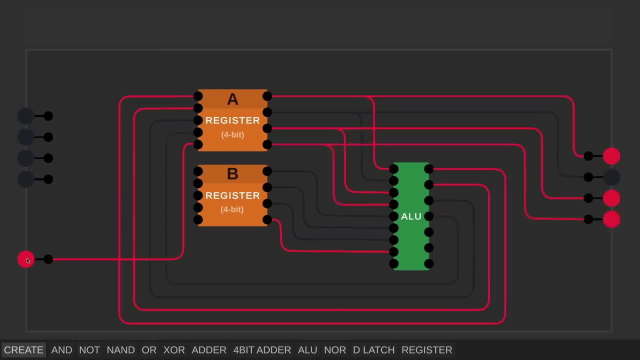 And enable it. Things have gotten a little out of control. I just wanted to store the result of 3 plus 1 in the A register, which, to be fair, it did, but then, a few moments later, the ALU calculated the result of 4 plus 1, which then raced around. 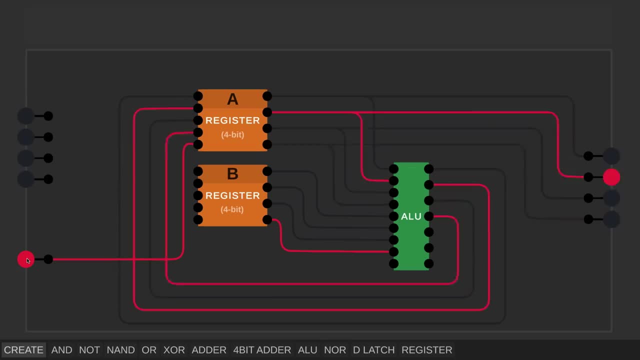 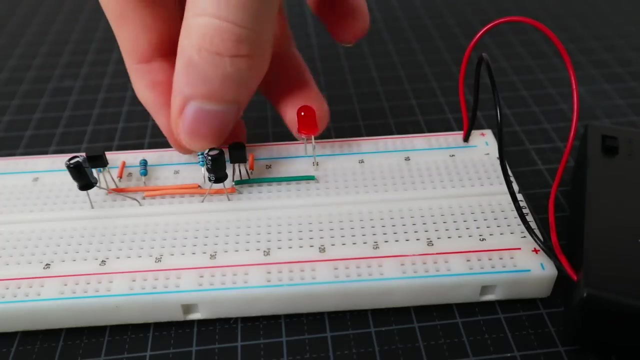 and overwrote that value. and then the same thing happened with 5 plus 1, and so on. So to capture just the first result, I'd need to turn the store signal on and off with impeccable timing. It works reliably, so we're going to need a bit of help. 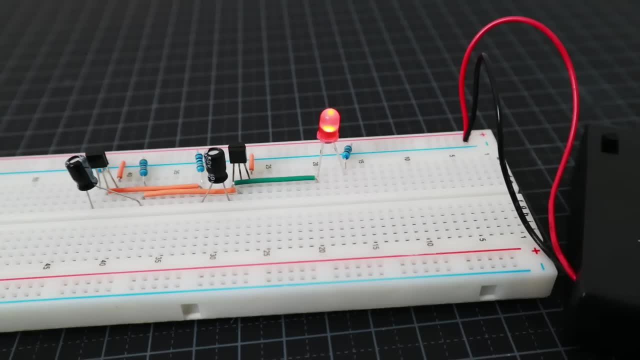 To the rescue comes the clock, which generates a signal that cycles endlessly between 1 and 0, also called high and low- at some steady pace. This is going to help us synchronise and coordinate everything that goes on inside the computer, and we'll pay more attention to it later on in the series. 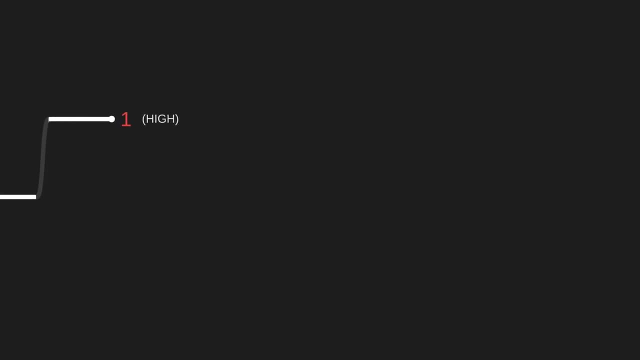 But essentially, during the flat parts of the clock signal, we want to do nothing, Because the speed of the clock is carefully determined so that this allows enough time for even the slowest signals in the computer to get wherever they're going and let everything. 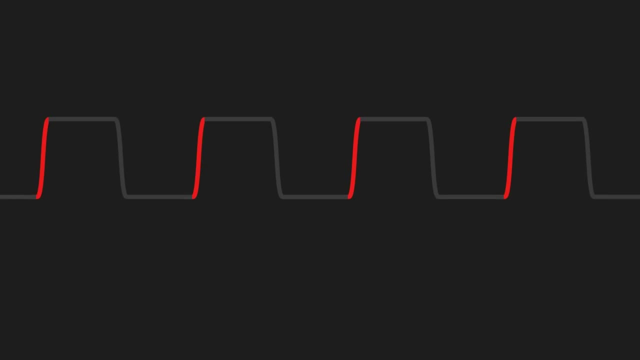 settle into a stable state. Then in red here we have what is called the rising edge, which is the very brief moment in time where the clock signal transitions from low to high, And then we also have the falling edge, where it transitions from high to low. 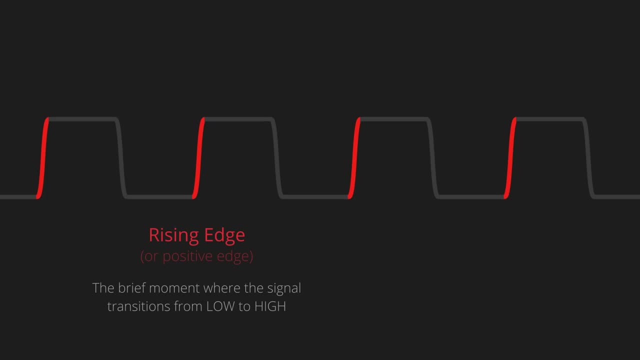 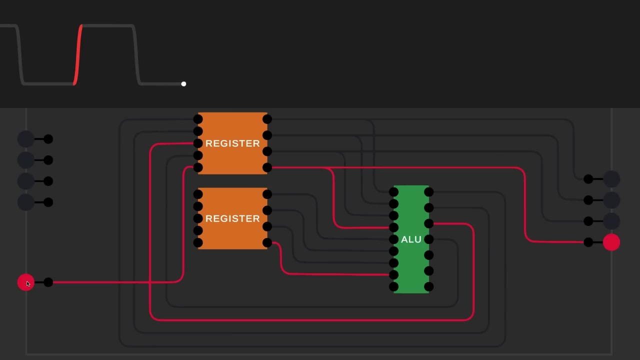 We can pick one of these edges, let's say the rising edge, and decide only to store data into memory at these moments. So if we can implement this, then in our setup from before, it would be storing the data at a controlled time interval instead of just as fast as it possibly can. 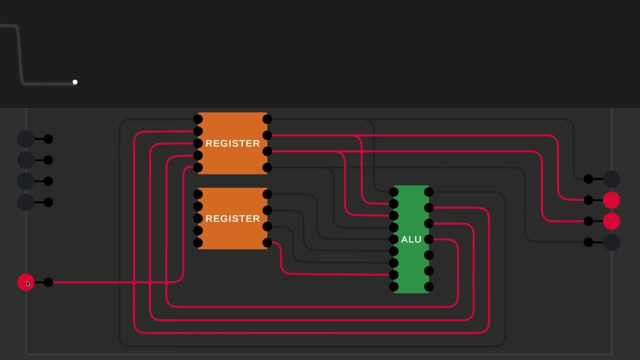 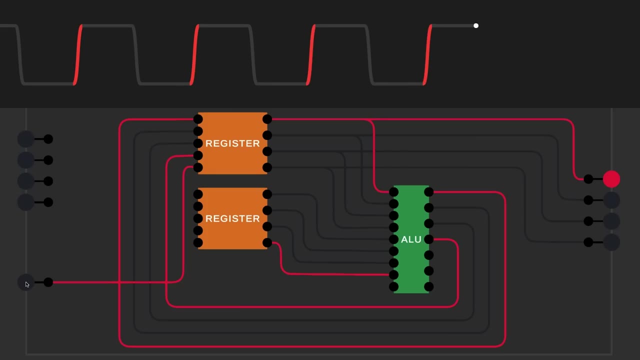 This will give us some breathing room to set things up between those rising edges, like turning off the store signal, for example. if we wanted to stop storing the data, That would be really helpful. so let's take that data latch rebuilt and try modify it. 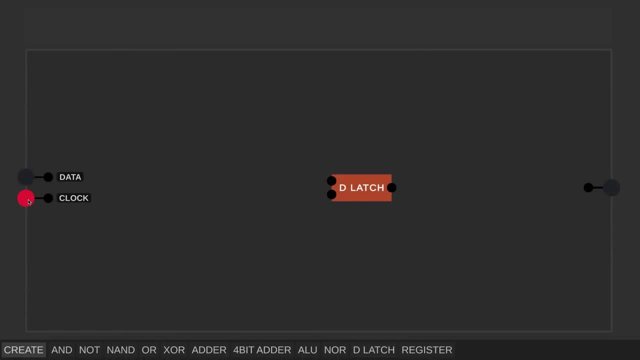 to only store the data when this clock signal here, which is the rising edge, is stored. So let's take that data latch rebuilt and try modify it to only store the data when this clock signal here, which is the rising edge. But for now I'm just controlling it manually so it goes directly from low to high. 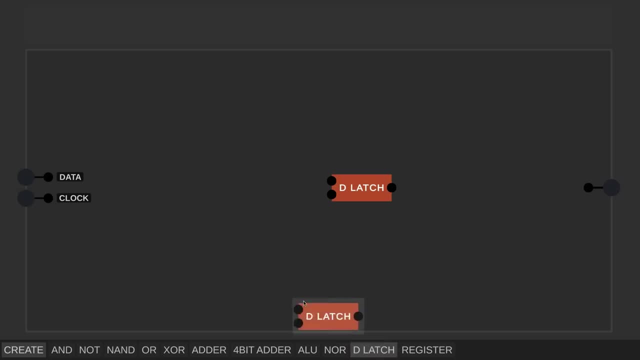 Now, there's actually a number of ways of achieving this, but I'm going to take an approach that uses two latches. The first latch stores the data only when the clock signal is low. Then the second latch copies whatever data is in the first latch, but only when the clock 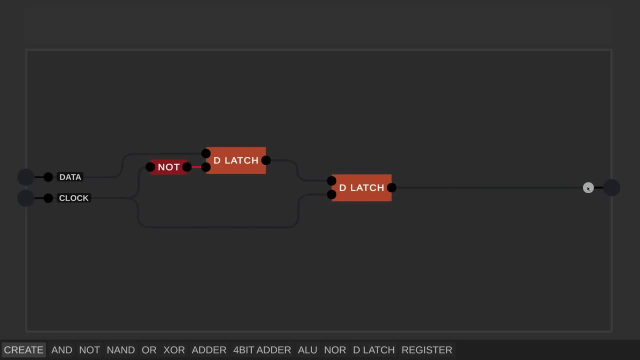 signal is high. Let's test this out. At the moment the clock signal is low, So I can change the data, but the output over here isn't affected. That data is, however, being stored in the first latch. If the clock signal were now to go high, we can see the output has changed to 1,. 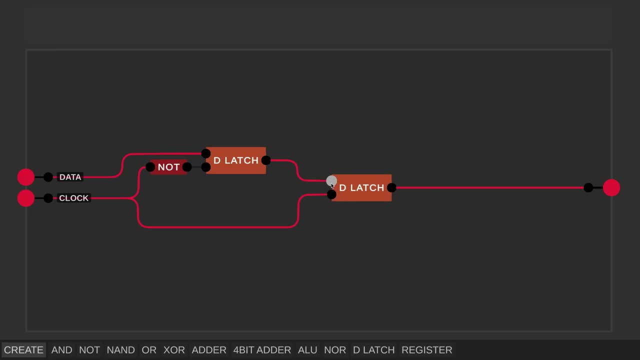 because the second latch is now allowed to load the value from the first latch. Again, changing the data does nothing because we're no longer storing it in the first latch, which is where the second latch gets the data from. So hopefully it's clear how this simple. 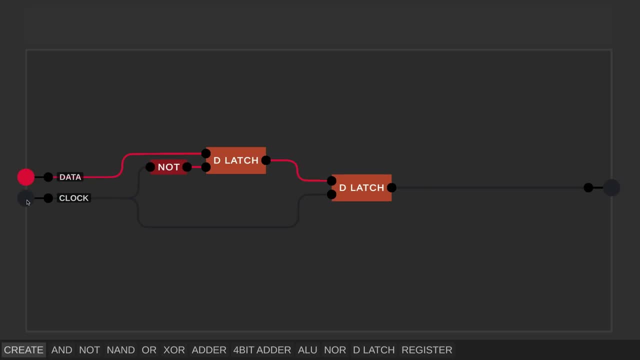 little setup achieves what we wanted: only storing data on the rising edge of the clock. What we've created here, by the way, is called an edge-triggered data flipflop. The trouble with this flipflop, though, is that it stores the data on every rising edge. 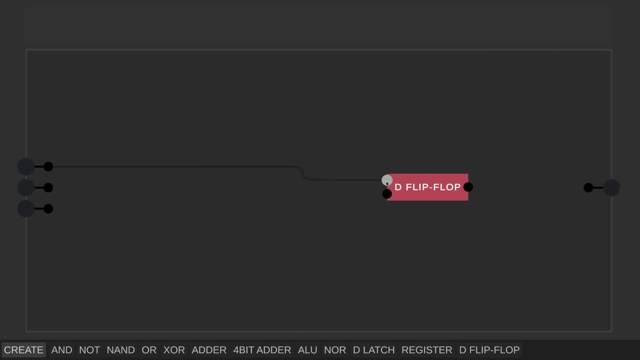 there's no way for us to tell it to stop storing the data. So over here I have a data and clock signal like before, but I've also added a store signal. The easiest thing to do would be to use an AND gate to modify the clock signal to be low when the store signal is off. 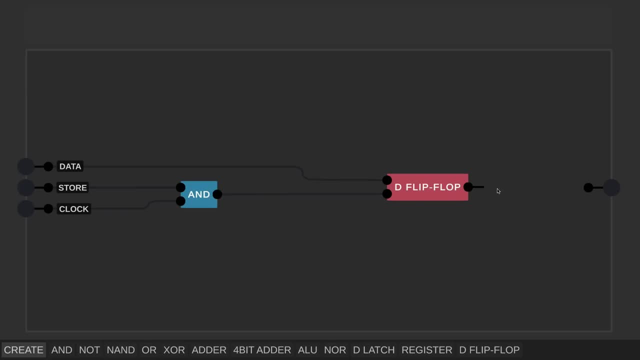 and, of course, if the clock signal remains low, the flipflop won't store the data. So, for example, I could put a 1 on the data signal and cycle the clock, but nothing happens because the store signal is off. If I turn that on though now, the data will be stored on the next rising edge. 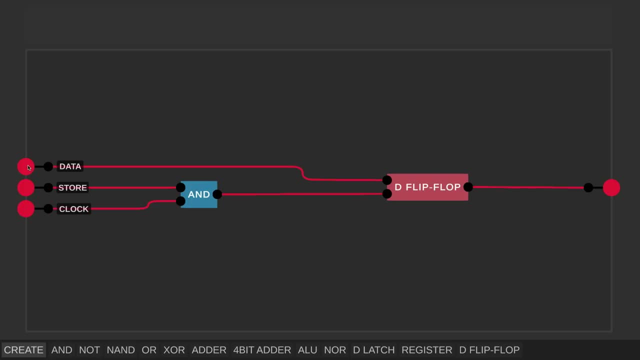 This setup does have a little defect though. For instance, if I change the data to 0, and turn off the store signal, the flipflop thinks the clock signal is low right now, although the real clock signal is still high. If I then turn the store signal back on, the flipflop will think the clock has just. 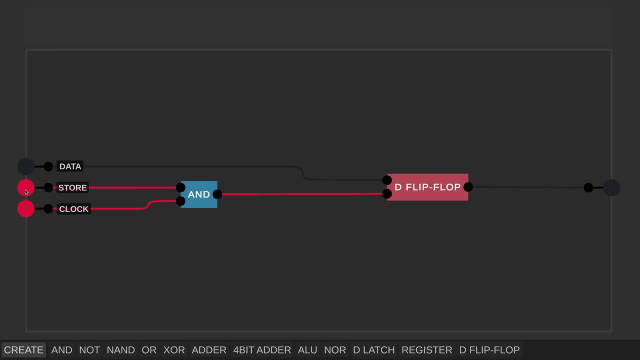 gone from low to high, and so it'll store the data at the wrong moment. This makes me a little uneasy, so let's go with a slightly more convoluted approach that doesn't have this issue. I'll give the flipflop the unaltered clock signal this time, and instead. 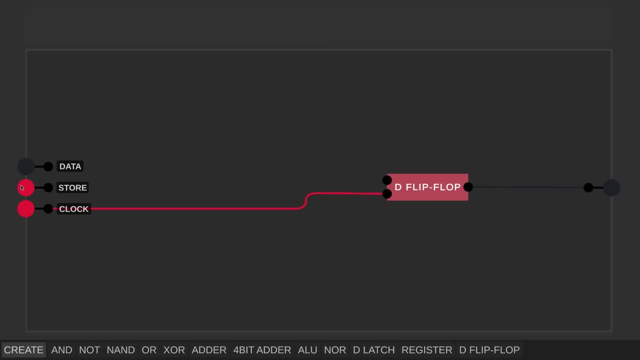 we're going to modify the data input on. we want to use this data input over here, but if the store signal is off, we'll instead take whatever is currently stored in the flipflop and just put it back in. To do this, we'll need 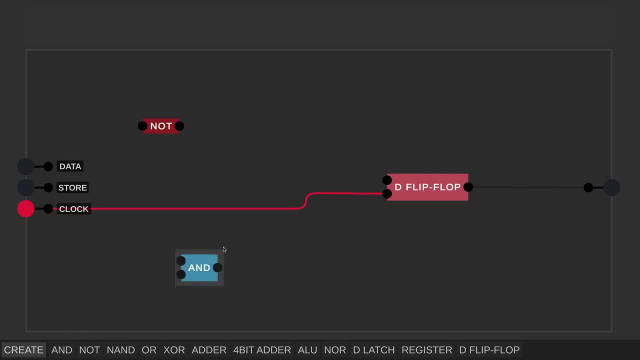 to build something called a multiplexer, and for that we'll need a NOT gate, two AND gates and an OR gate. The two bits of data we're choosing between go into each of the AND gates, and we want to choose this one if the store signal is on and the other one if the store signal is. 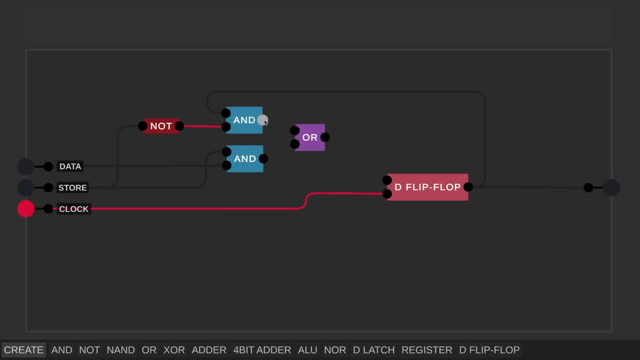 not on, Then whichever is chosen, we want to output it on a single wire, so that's the purpose of the OR gate. Let's give this a quick test. So I'll try putting a 1 on the data signal, but as we designed, with this store signal off, it's simply taking the 0 that's currently stored. 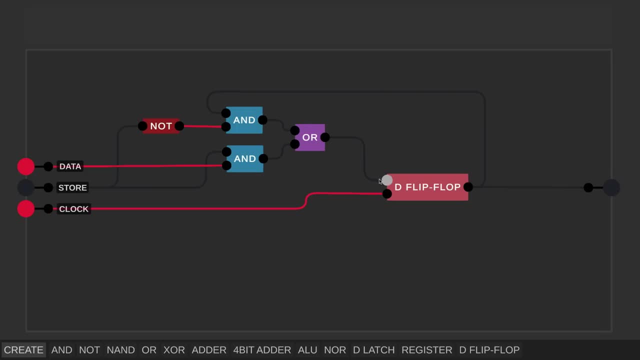 in the flipflop and feeding that back in, and so nothing changes when we run the clock. If I turn on the store signal, though, now it will actually store the new data on the rising edge of the clock. As a final test, I'll set the data signal to 0, turn off the store signal. 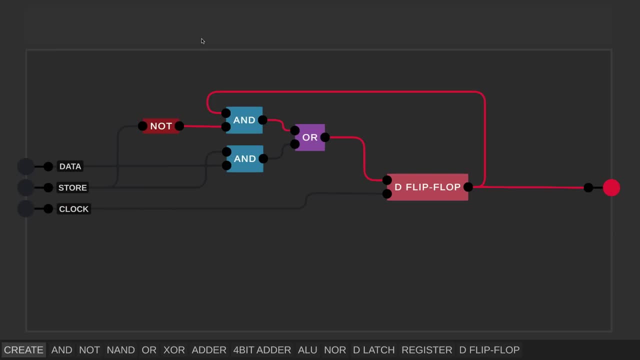 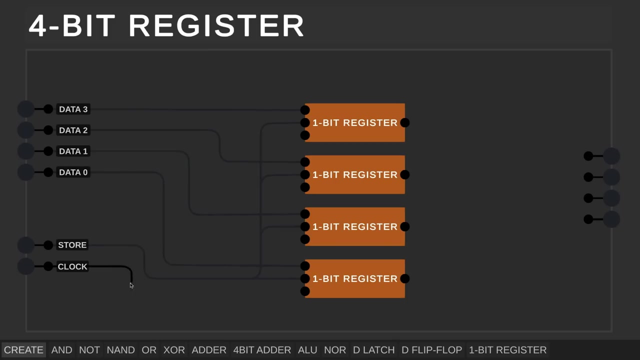 and make sure that works as well. Okay, I'm going to call this a 1-bit register and we can use it to make an improved version of the 4-bit register from earlier. Okay, let's see this in action quickly. I'll set some arbitrary data. 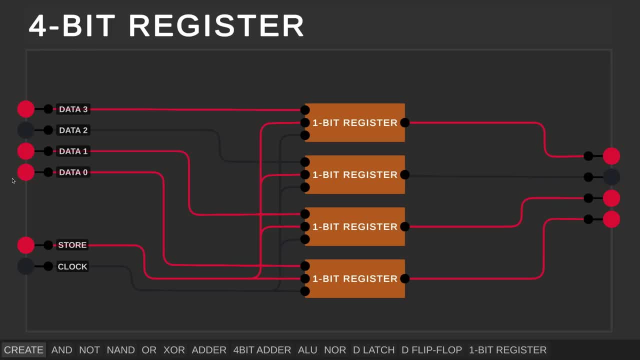 turn on the store signal and then pulse the clock to load that in. I'll set some different data then, and let's try it with the store signal off this time, just to be sure that that's working, which it does seem to be. 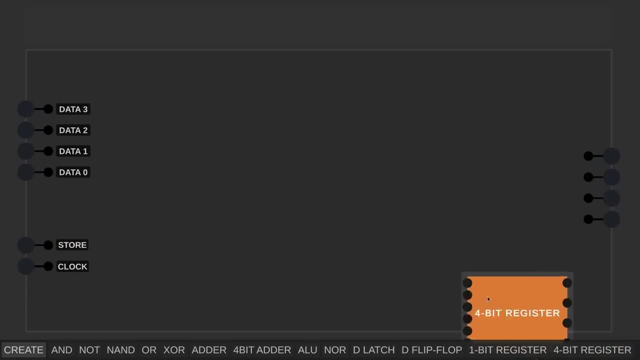 Alright. so remember our setup from earlier. that was running out of control. Let's set that up again, but using our fancy new clock synchronized registers. So I'll load some starting data into both of these, let's say 5 into the A register. 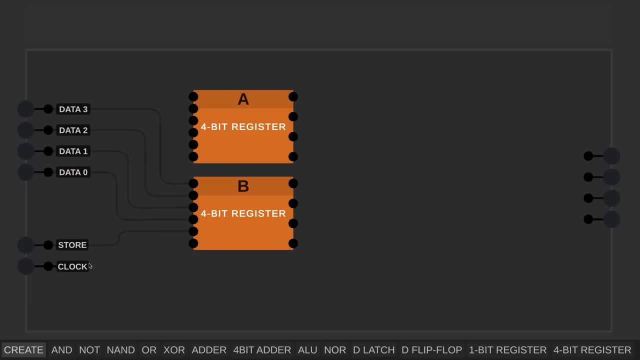 and then I'll connect the inputs up to the B register and store- maybe 3, in there, Like before. I'll then hook these both up to the ALU to add their values together and send the result back to A. Finally, let's connect the store and clock signals up to the A register. 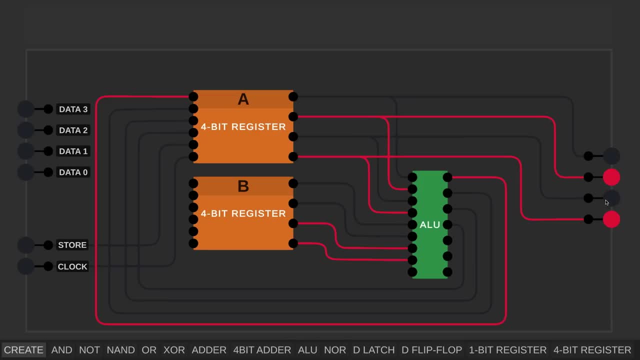 So at the moment it's outputting 5, but I want it to load in the result from the ALU So I can turn on the store signal over here and then, when the clock signal goes high, we can see the result has been loaded in, because the output has changed to an 8..